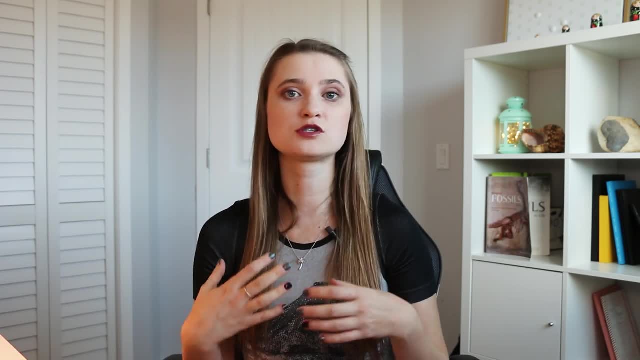 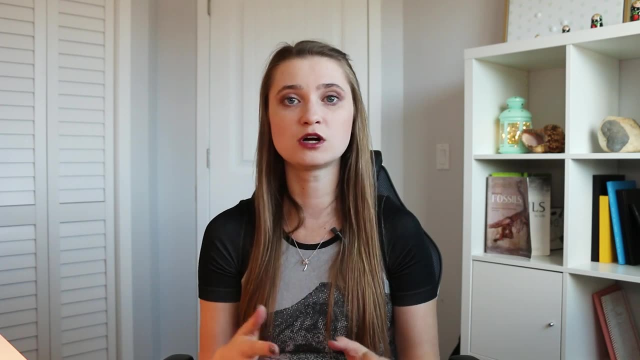 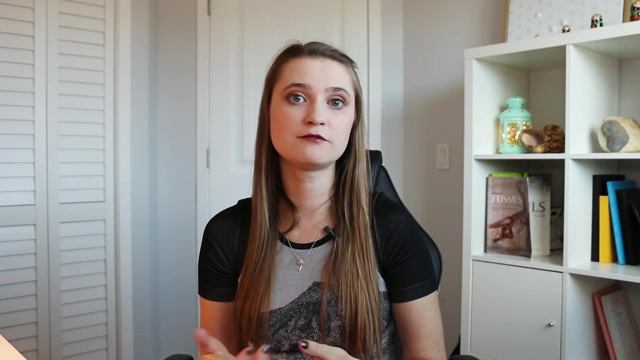 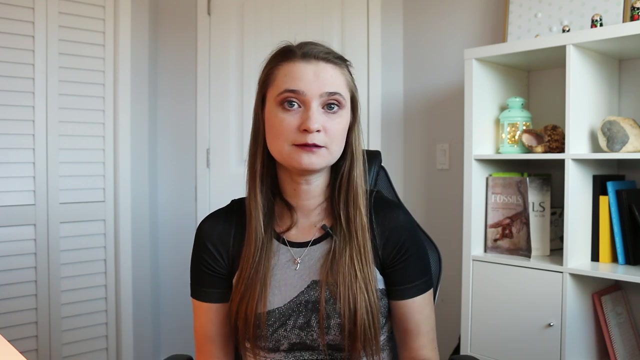 mining companies, oil and gas companies looking for resources. They can also work for environmental companies, construction companies and government bodies doing geological surveys or do academic research. What are main job responsibilities of geologists? Well, that's basically collecting data from the field, from geological sites, for further analysis, for further studies, do mapping to. 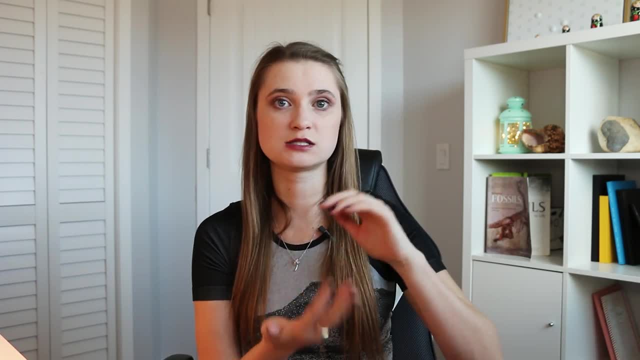 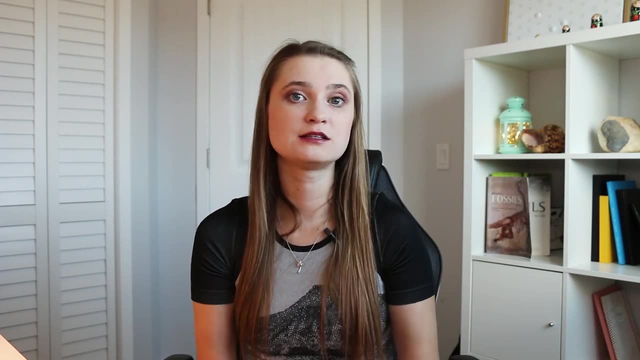 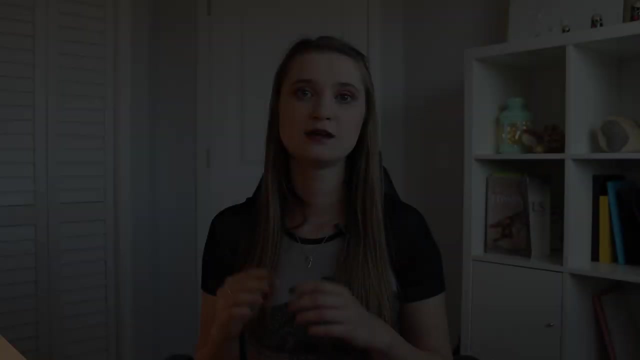 interpret both the surface, the topographic maps, as well as the internal maps, to interpret the underground layers and as well as to communicate the findings to managers, to stakeholders or just general public and do scientific research. Now let's look at geophysicists. 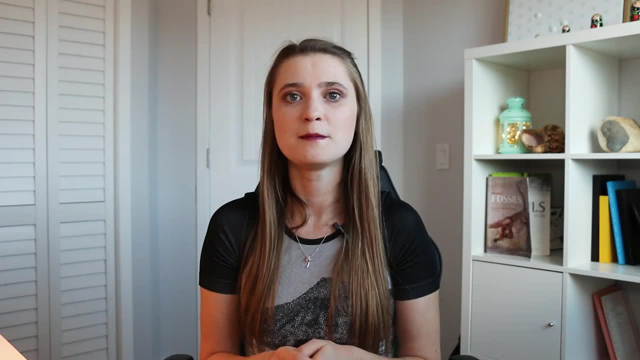 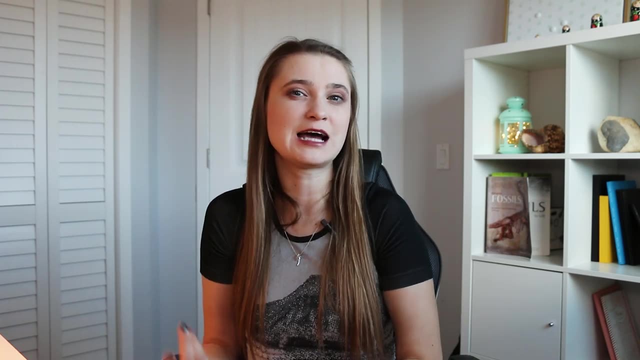 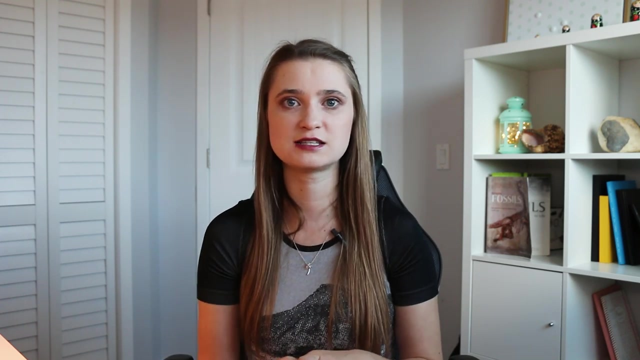 Well, geophysicists do a lot of many things that geologists do, but as a general rule of thumb they don't do as much field work as geologists do and they collect a different type of data. A lot of geophysicists collect seismic surveys, gravity resistivity surveys they work with 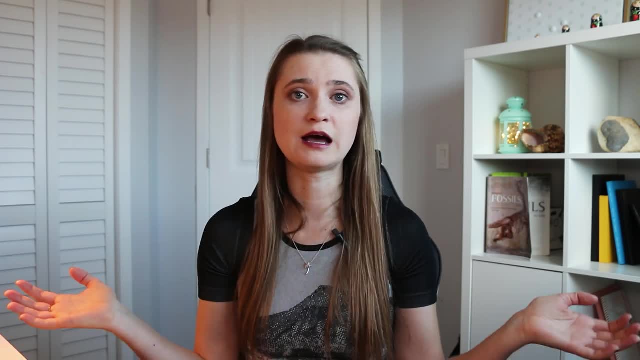 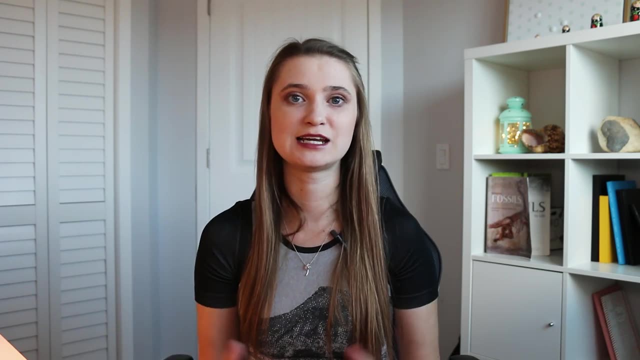 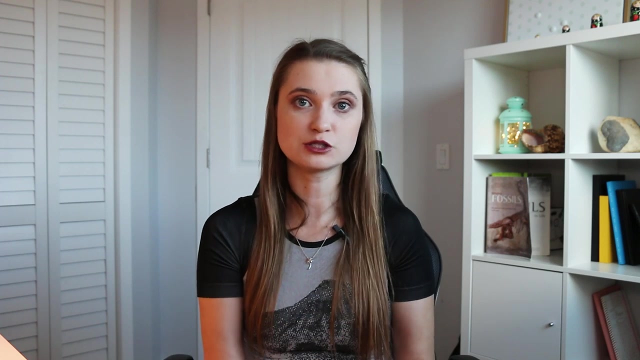 gravity data and magnetic data and often after they collect the data, they sit in front of a computer and do a lot of crunching and a lot of modeling and analyze the data to support a geological either theory or to support geological finds for resources. Geophysicists can also work. 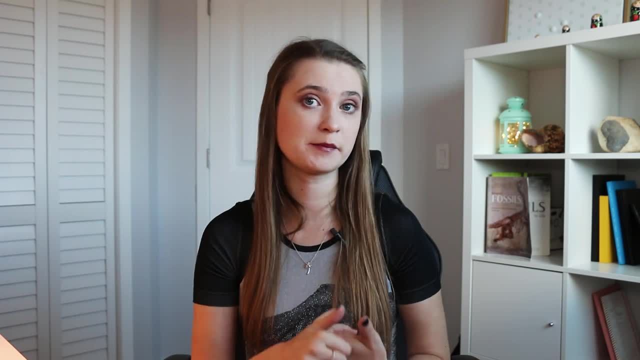 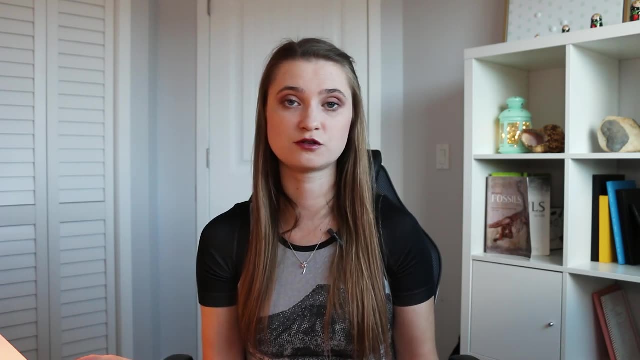 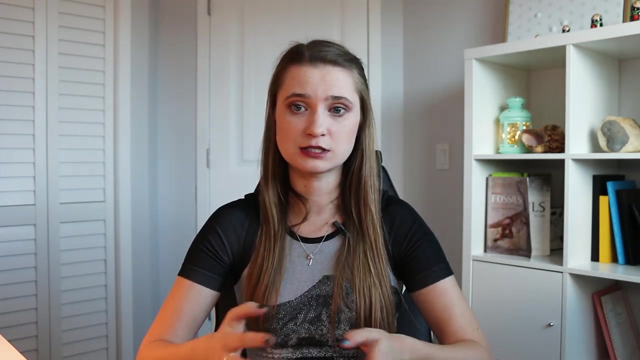 for mining and oil and gas companies, for resource companies, for geophysicists, for environmental companies, construction companies and government bodies as well, as well as do scientific research. So the overlap is huge. Now more calculations and modeling is done by. 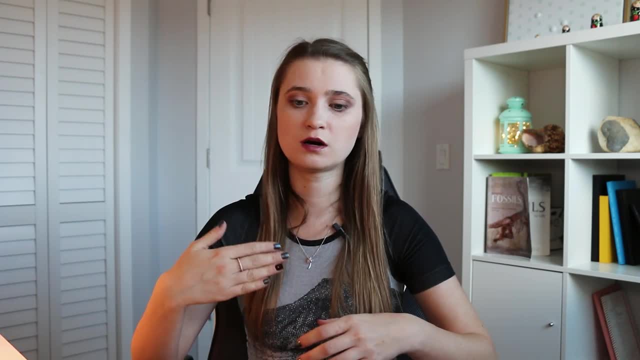 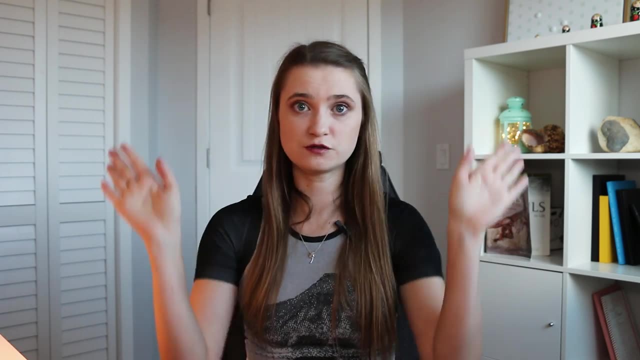 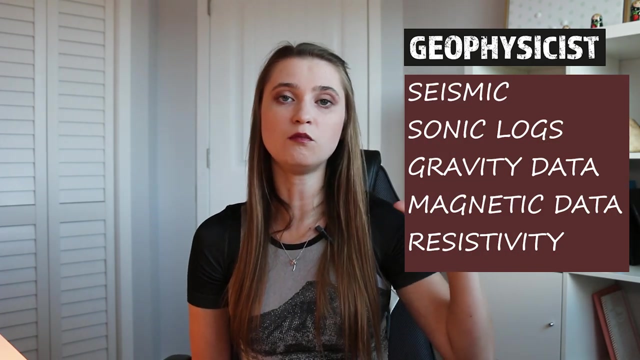 geophysicists, whereas more field work and more stratigraphic analysis mapping is done by geologists. Now to compare the two, it's nice to visualize, So I created the table. So geophysicists are more computational, they're more analytical and they work more with seismic data, sonic logs. 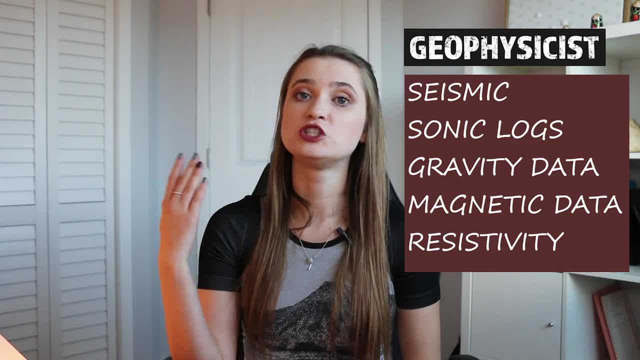 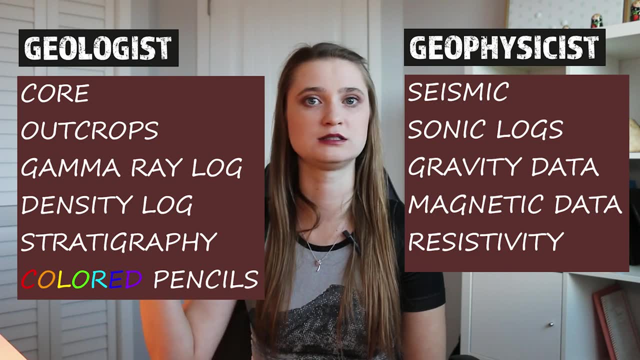 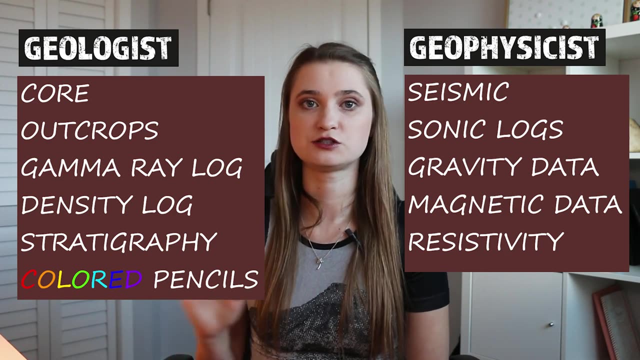 gravity and magnetic data, as well as resistivity logs. Geologists, on the other hand, are more interpretational and observational, and they often work with data that came from core analysis from outcrops, gamma ray density logs and stratigraphy, and geologists use a lot of. 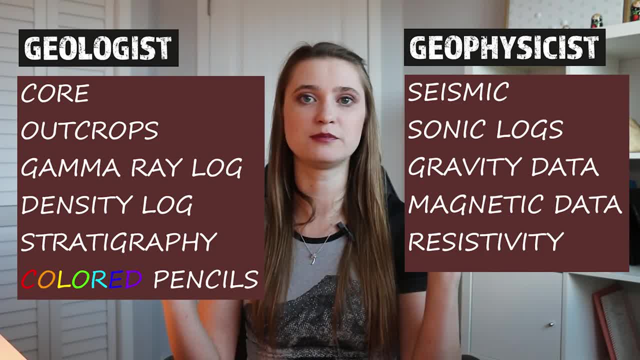 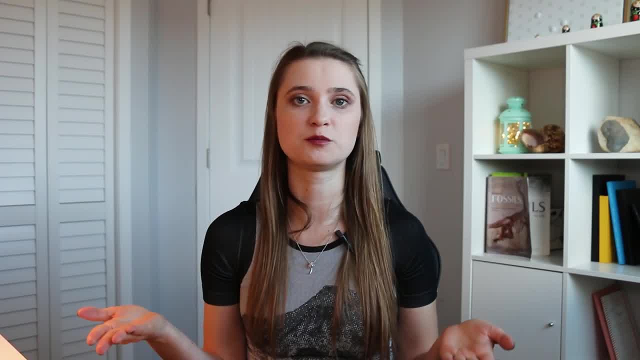 color pencils, But as a whole they're more computational, they're more analytical and they, as you can see, both professions work towards the same main goal and that's to create a model of the earth and to interpret the earth. Now, from personal experience- and I worked for an oil and gas company. on our team we always had a geophysicist. Geophysicists made a little bit more money On average. in Canada, the average salary of geophysicists are around $75,000 a year. That's an average, so there's a huge range between. And geologists on average make around $69,000 a year. However, even though that might sound lucrative, there is way less geophysicists than there are geologists working on a team usually, So in the company I used to work for, that ratio would often be around 10 to 1. So 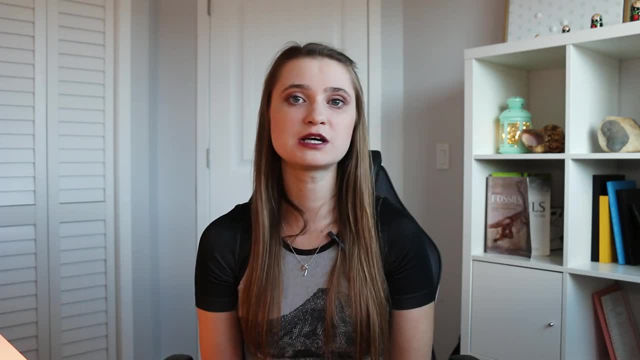 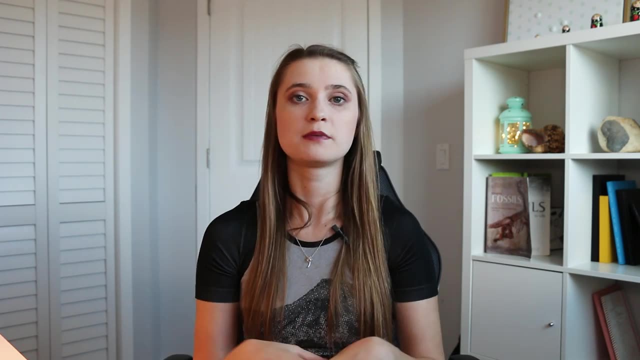 for every geophysicist there would be 10 geologists, And that's because, as a geologist, I not was only analyzing data, I was not only mapping the area that I was given too, But I was also responsible for mapping. I was responsible for finding future drill locations. 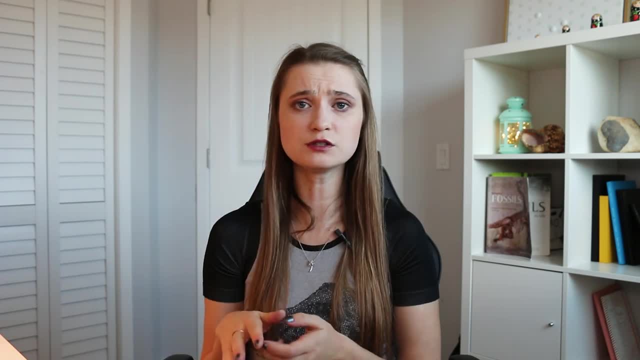 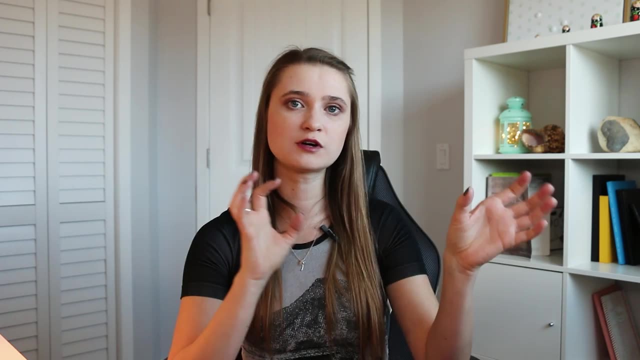 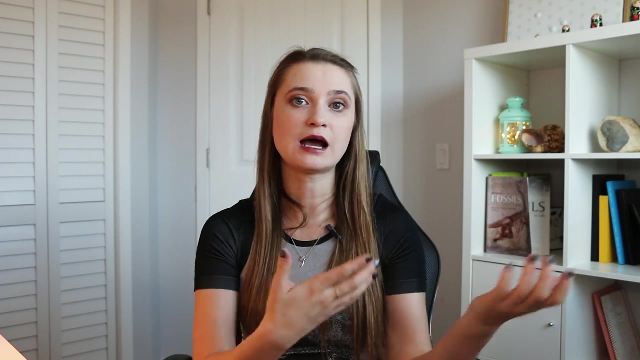 I was responsible for creating those drill schematics and I was responsible for overseeing the drilling when the drilling rigs were actually drilled. So there was a lot of components to my job, not just strictly science and geology, Whereas geophysicists that I worked with 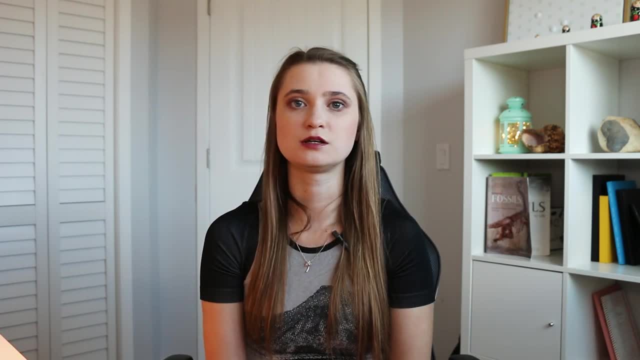 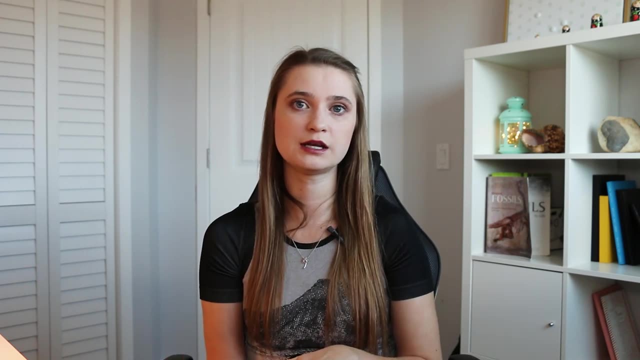 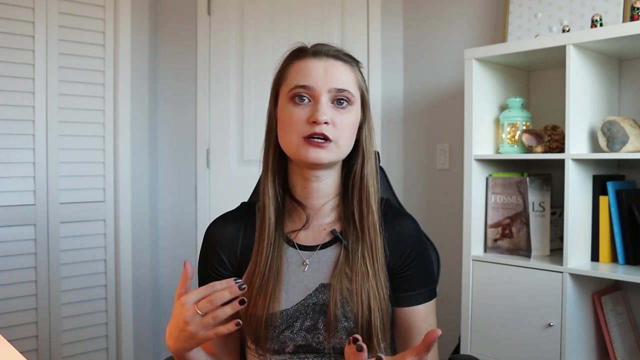 he or she would be responsible for doing seismic surveys or like micro-seismic sometimes we did in some wells, and then putting it into one big model, creating a 3D model, maybe using sonic logs and resistivity logs as well as the seismic surveys, and then integrating 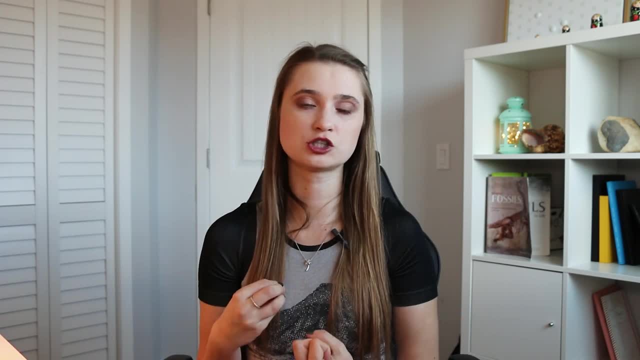 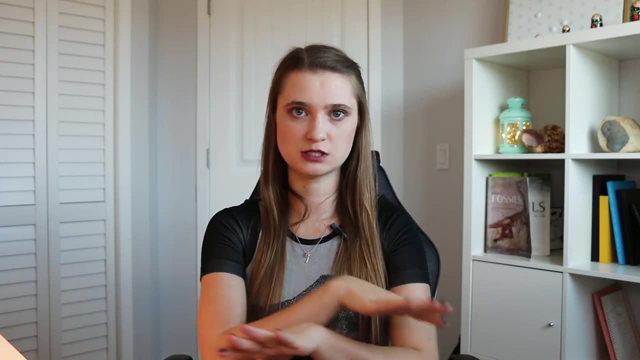 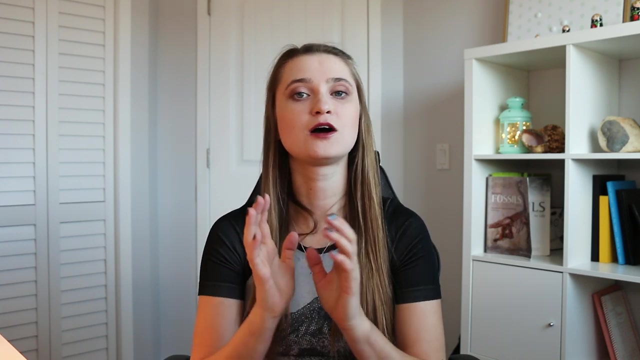 that data analysis with my geological interpretation to create one big model, And so geologists would cover smaller areas where geophysicists would cover one large area. So because there's less geophysicists, it's much harder- It's hard- to find a job as a geologist, but it's much harder to find a job as a geophysicist. 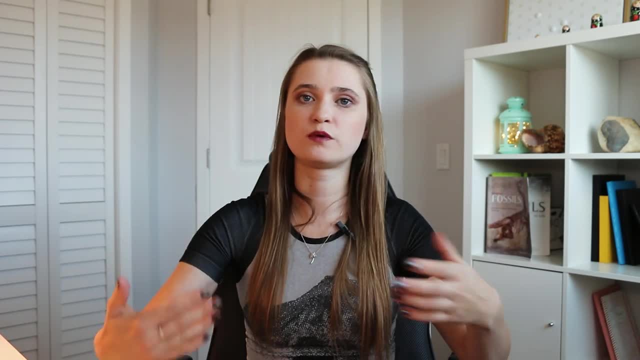 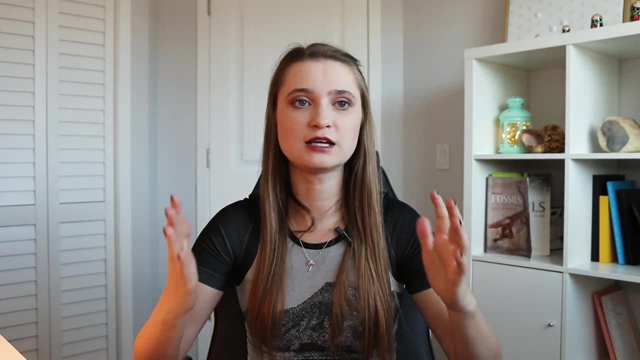 as a rule of thumb, That's not everywhere and that depends where you are. So with that, I wanted to address the question which one is better. Well, neither is better. They're different, but they're both equally important. Petroleum companies especially. they need both. 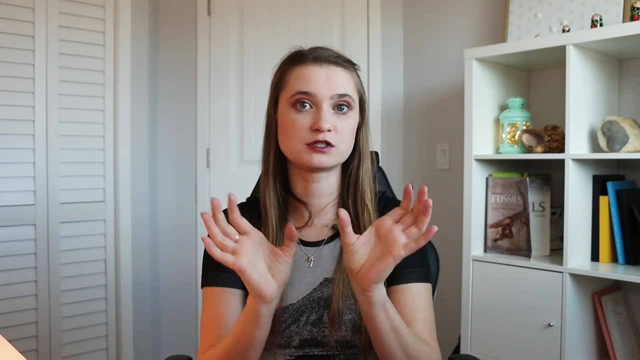 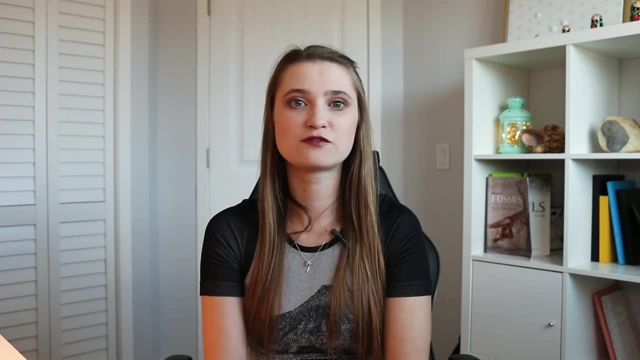 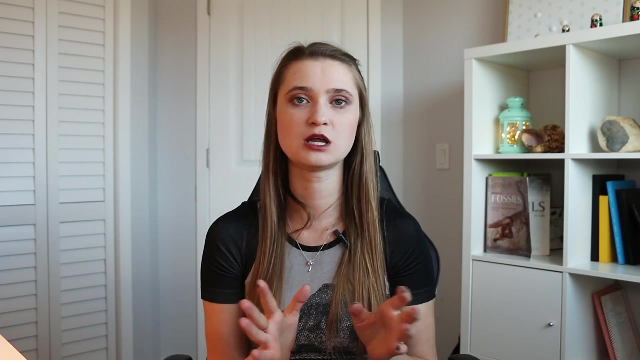 professions as well as mining. They have different set of skills. Now I also get asked: what should I do? And that comes from: don't take my opinion as an advice what you should be doing. you should be looking at your situation. But in general, I would say most companies would require. you to do master's regardless. So it's good to have a general geoscience or geology bachelor's and then do master's in geophysics. And that's because in my geology program I was required to be a geophysicist And very early on I realized for myself that I don't want to be a. 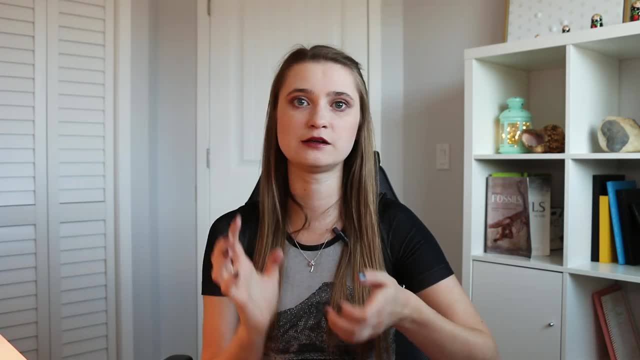 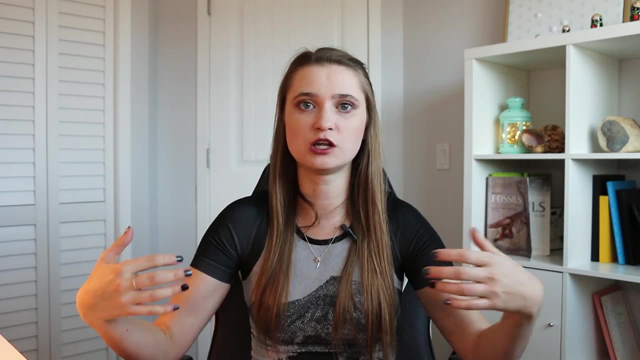 geophysicist. I'm not enjoying crunching data, sitting in front of computer modeling all the time. I want to be in the field, I want to do mapping, I want to do a lot of interpretation And I found like geology is more creative for me. but I'm just not very analytical. People that are 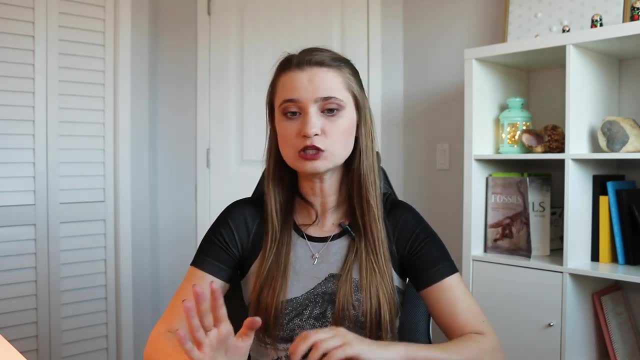 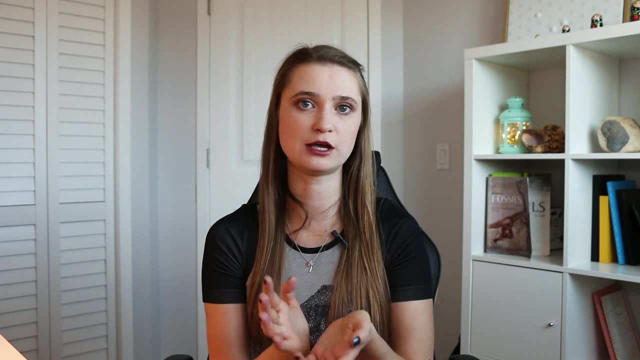 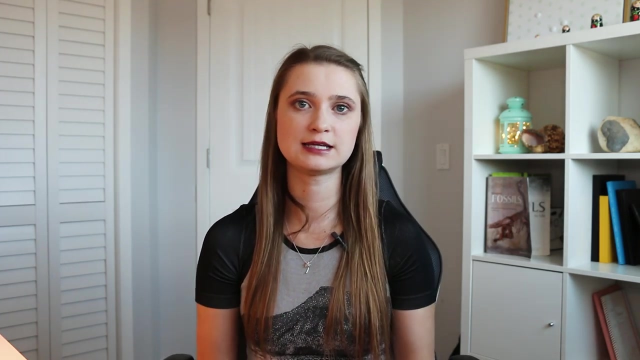 very analytical. they enjoy geophysics more. So if you were to do a general geology degree, you would do geophysics regardless, because most university would make you to take geophysics classes if you're in geology program And then you can decide what- if you like it or not, and take more. of those classes in your master's program. But having a geology-based degree would give you more opportunities to look for jobs Once you graduate with your master's. you can apply for both geology and geophysical positions. Also, from my own experience, all of my friends that are geophysicists. 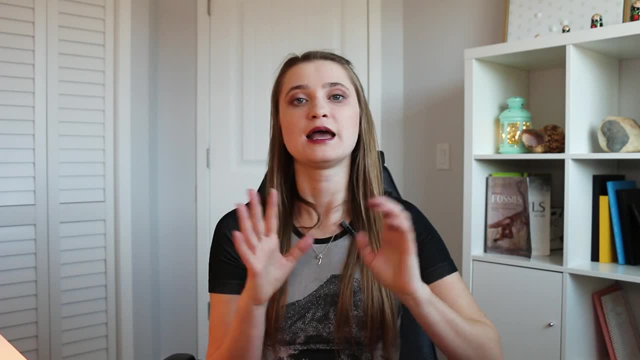 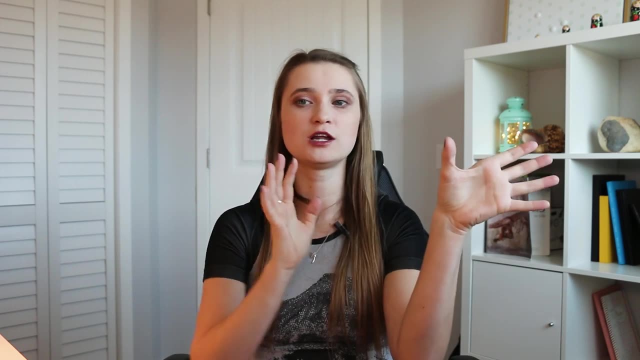 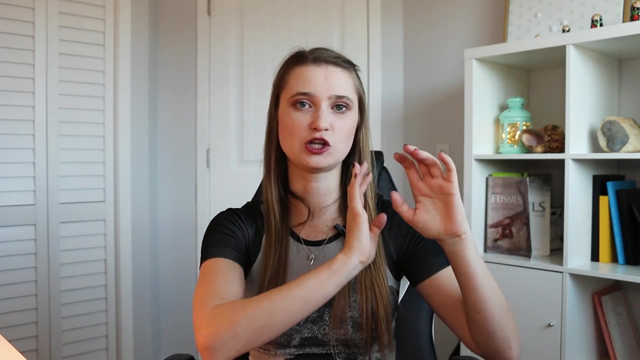 they are more analytical, They enjoy math more, And I always think about geophysics being kind of like this middle, happy middle- between geology and engineering, Whereas geology is on one end of the spectrum where it's interpretive and there's a lot of sort of not guessing. 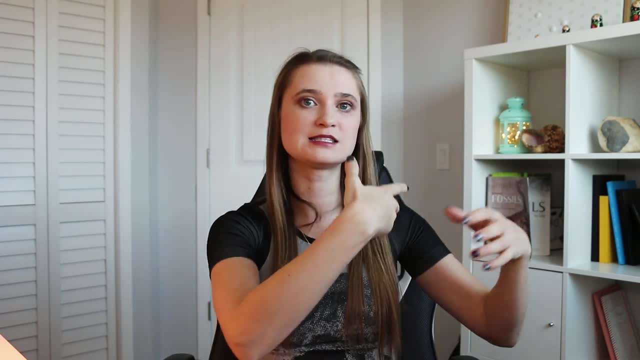 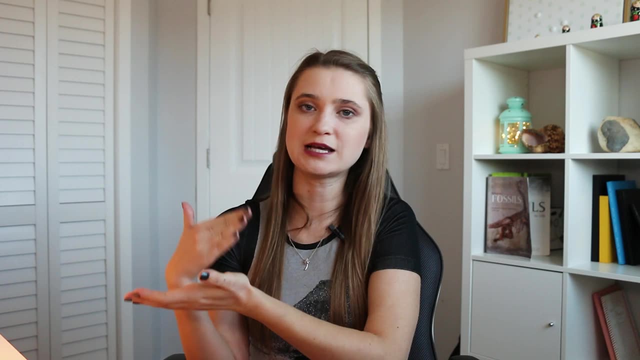 but scientific guessing goes into it And there's a lot of things that are open to interpretation. Engineering is on the other spectrum, whereas everything is very precise. They use precise numbers to do their models And, yes, they do various models, but it's very 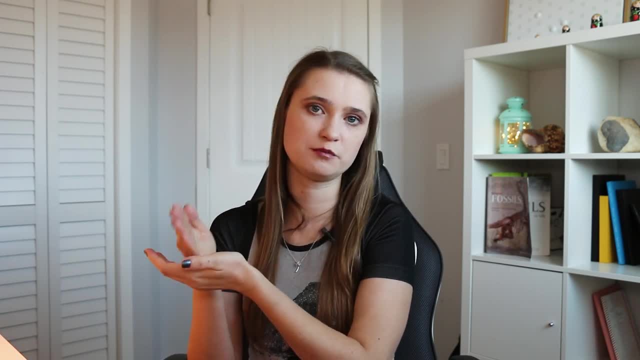 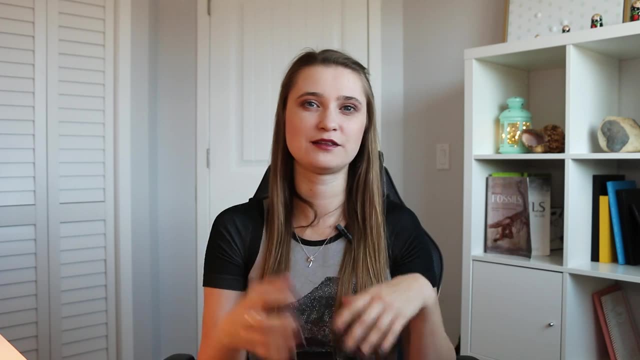 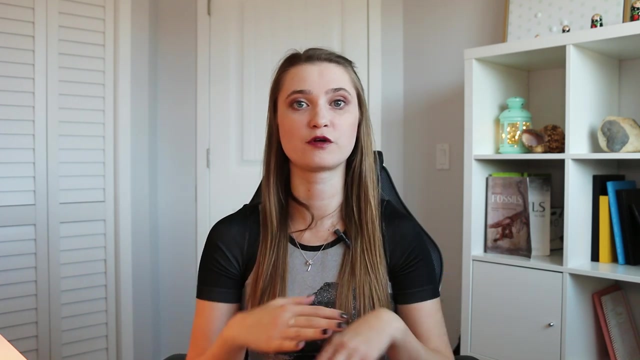 very analytical and very- it has to be very precise. And geophysics, here in the middle, where they do work with data. they're more analytical than geologists, on average- not always, But they also have a lot of room for interpretation for their surveys, for example. 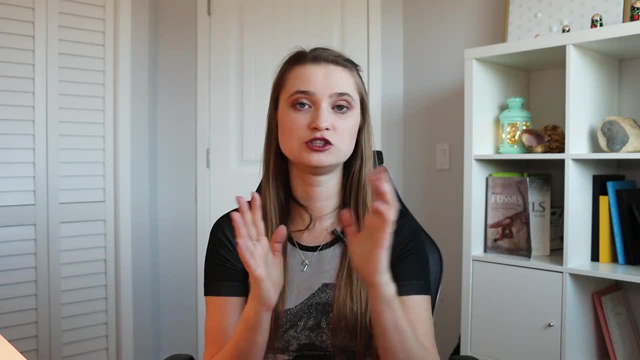 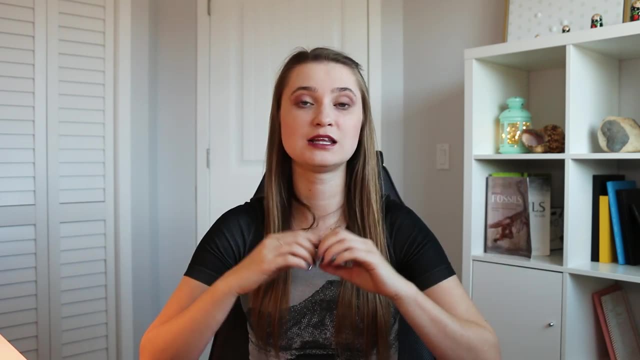 Now, depending on what field you're working in, geology and geophysics can be very, very much alike or they can be very different, And a lot of, for example, in petroleum world, especially- that's because that's what I know- for smaller companies. 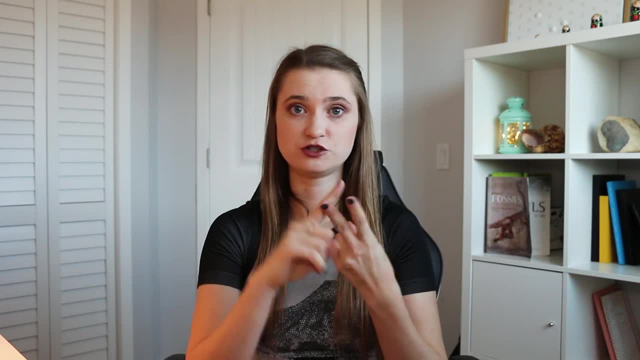 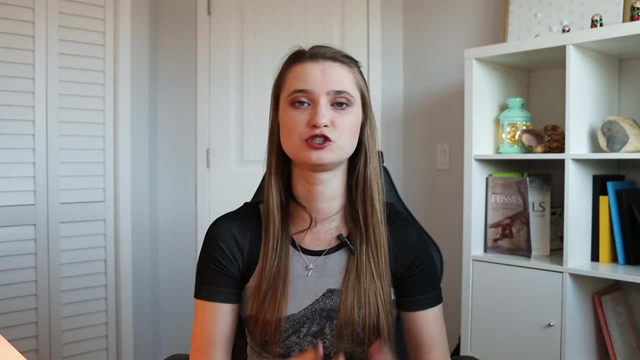 a lot of the time one person would be doing job of a geologist, geophysicist and a petrophysicist, So it's nice to know a little bit from each field. Because I took geophysics classes at university, I have enough knowledge to understand seismic surveys.